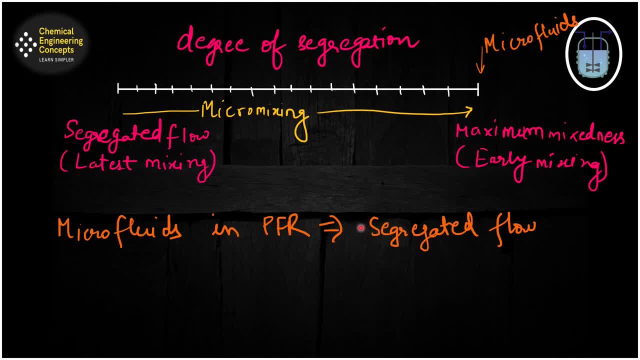 will not give you the actual value, or we should say the correct value of conversion. So we should have to define the mixing patterns also. Here you can see the scales of the degree of segregation. These are the degree of segregation scales for the micro mixing. So on the one side we can see that we have the segregated. 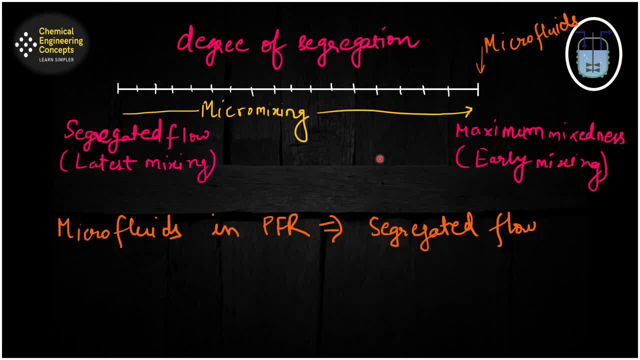 flow, where we have the latest mixing, and on the other extent, we have the maximum mixedness model, which is the early mixing, and the micro fluid lies on this side. So, guys, it will depend on the type of mixing we will have. So we cannot be on this for the real reactors. 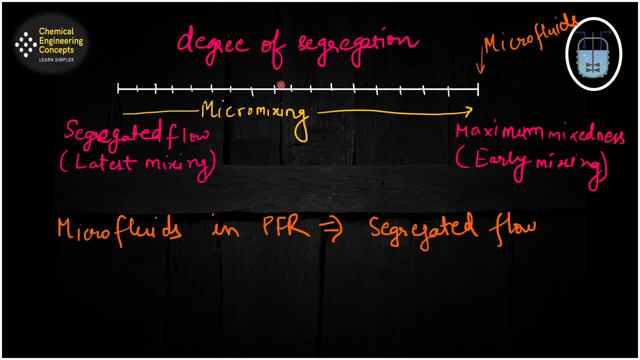 We cannot be on any one of the extent and we will be on any of these intermediate scales. We will have these intermediate values of micro mixing. Now, when it comes to micro fluids in PFR, that is the plug flow reactor. So we have two extents: a plug flow reactor and 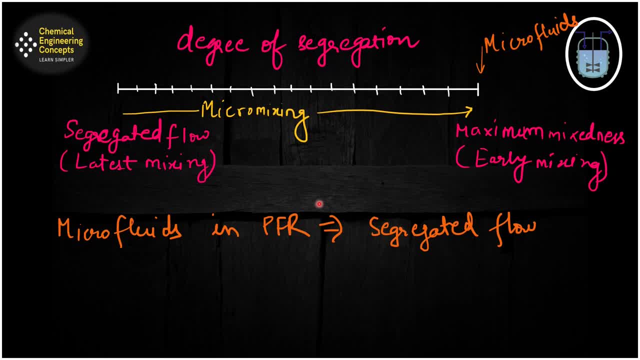 the mixed flow reactor, The micro fluid or the macro fluid or any of the fluid, will go to a plug flow reactor. that will give you a same conversion, Because we know that for a PFR, in a PFR, we have a n number of small batch reactors. and for the batch reactors, whether it is micro fluid or 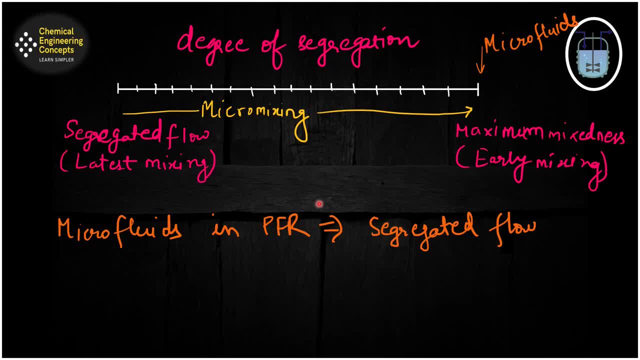 micro fluid. they will spent the exact same time inside the reactor and they will have the same conversion. So for the micro fluid, Even for the micro fluid, V chose mixed level of sm, 악, ph, dep vier, two extents al th applaud, mister phuар. 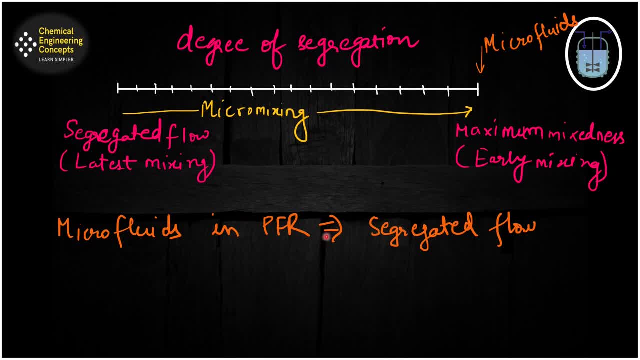 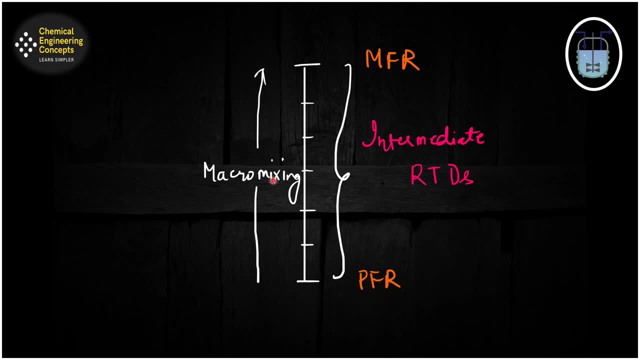 pas fluids in a pfr. we will have on this side right, that is the segregated flow now when it comes to macro mixing, right. so we have two extends that you can see here. first one is towards the mixed flow reactors and the other one is the pfr. so this lower end resonates with the left hand side of the 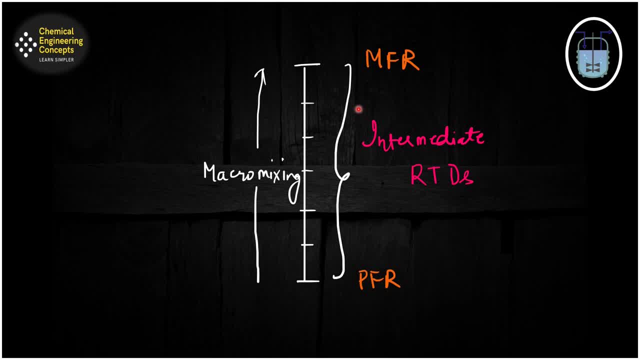 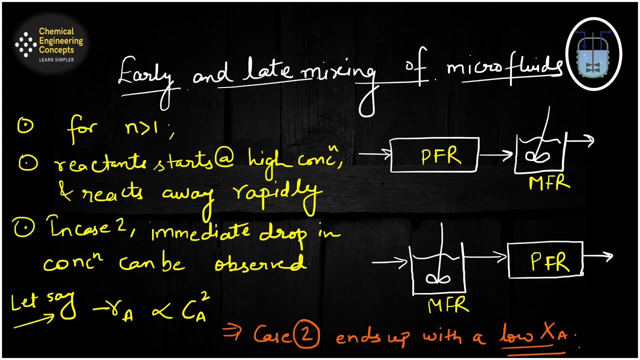 previous discussion, previous slide that we shown right and intermediate. we have some in in the mix. in the intermediate values we have some rtds, right residence time distribution that have to be taken under consideration right. so now let's uh understand about the earliness and lateness. 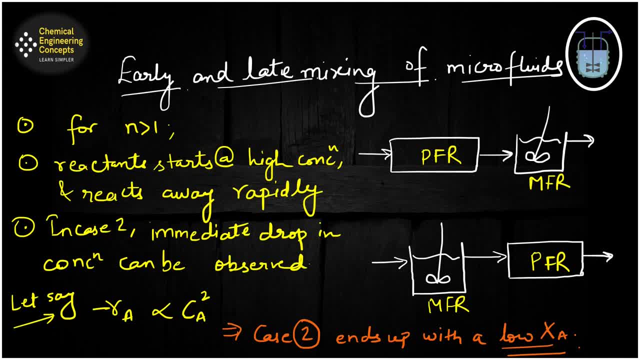 of mixing for the microfluids- okay, the microfluids that we are taking here. so here we have taken an example of our order of reaction greater than one, and two cases we have considered. first one is the pfr in series with the mfr, and the second case is all the opposite, one that 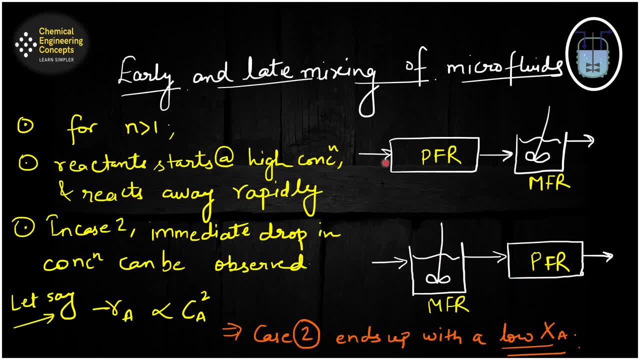 is the mfr in series with a plug flow reactor. right. so in the for the first case, if i should say for the first case, since we have a pfr on the start and mfr on the second, on the second half part, right, the in this when, when the reactant enters this system, this first system, the reactant 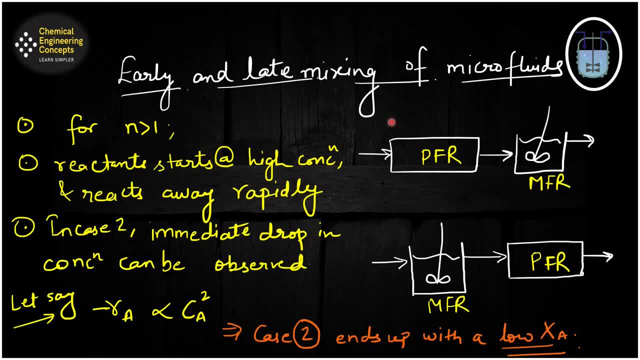 starts at a very high concentration, obviously, and it will react away rapidly. right, it will react away because we have the order of reaction has to be two, okay, and the reaction rate is directly proportional to, uh, the concentration, the initial concentration, right, so it will react away rapidly. 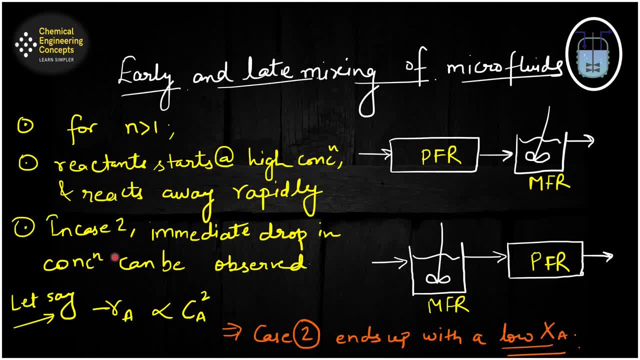 but, guys, if you see the case number two, okay, we have the case number two and because of the mfr on the first part, on the first half part, there will be an immediate drop in the concentration, okay, which you will observe. that's why. that's why. 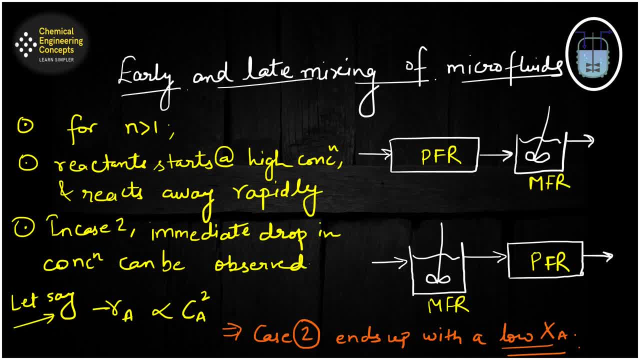 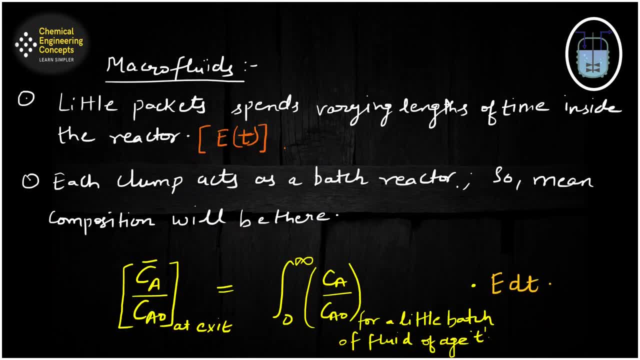 for the case number two, you will end up with a low conversion, right? so this mixing patterns is really very important when it comes to the type of fluid as well, right? so now let's consider the macro fluids, right so in the macro fluids, as i already told you, we have a small batch, batch. 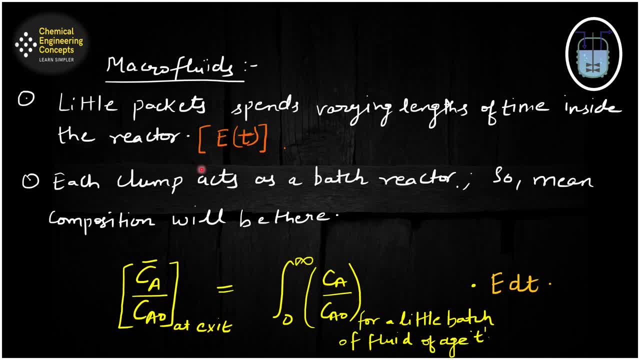 reactors, right, which we generally call as the little packets or clumps that will spend varying lengths of time inside the reactor. that's why, because they have varying lengths of time, they will have an rtd. hence the rtd function okay, so each clump will be acting as a batch reactor. 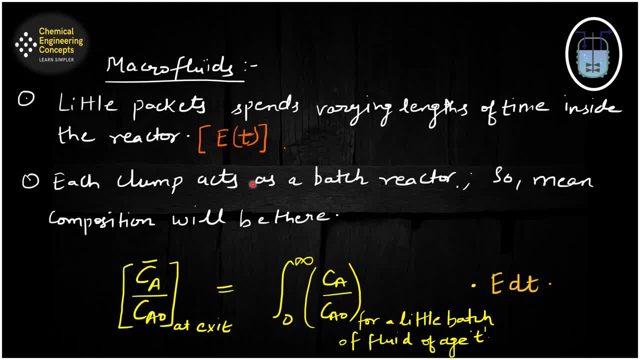 so, hence, there will be a mean composition, right, and because we have a mean composition there, you can see the mean composition that is coming at the exit. okay, and that i have calculated using this. okay, because we have different batches and we have to calculate the mean value of. 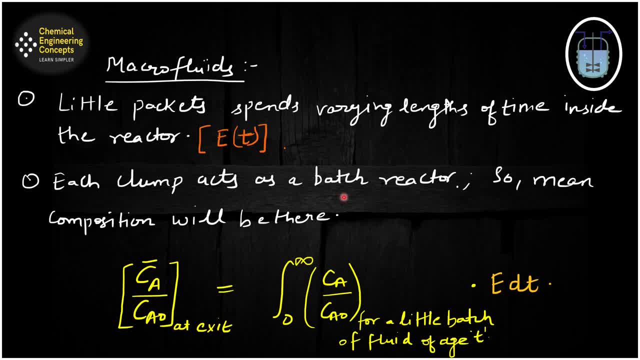 composition. so it will be the integration. okay, i have to take all the batches and integrate the average exit composition right. that will give me the mean composition multiplied by the residence time distribution function, because they have varying lengths of time that they are spending inside the reactor right, and multiplied by dd, because we have an. 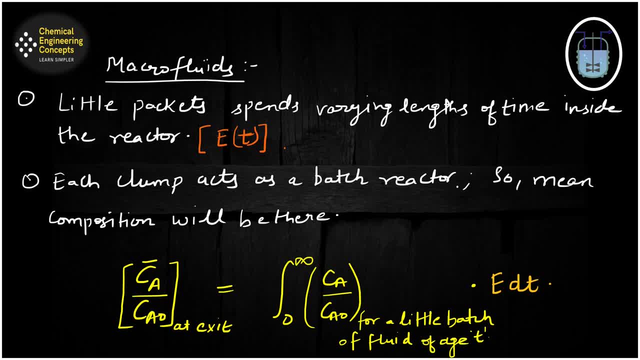 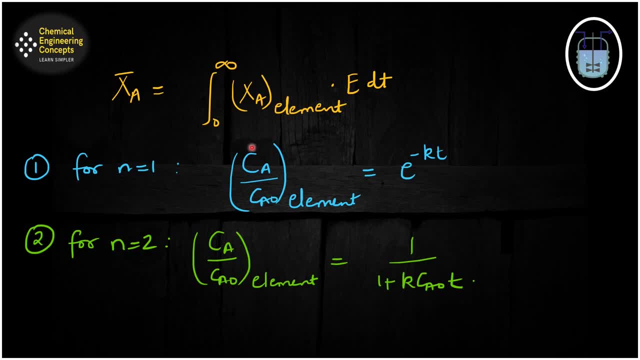 integration. right, so this will give me the mean composition at the exit. okay, we can write it in terms of conversion as well, mean conversion, basically. so it will include the uh conversion of each of the element. okay, the element i'm i'm just uh referring here, uh, as the different batches. 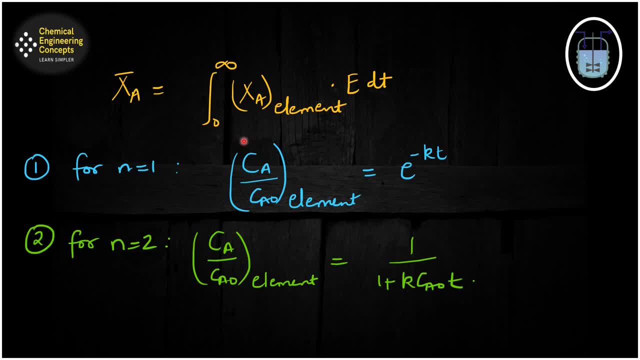 right, different batch reactors. now let's take an example of the reaction order to be one. for the reaction order to be one, we have this element, okay. so this element simply is: is, uh, the concentration ratio for one batch reactor? okay, when we have taken the order of reaction as one and we know 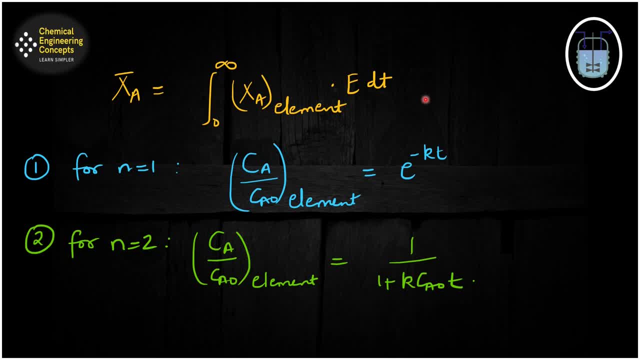 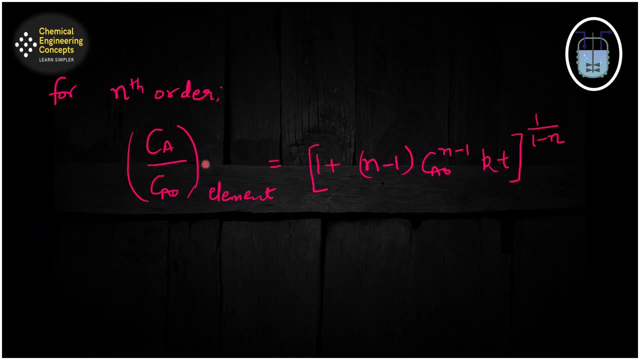 that it is exponential of minus kt right, and for the n equal to 2. okay, this will, this is these all, uh, you know from the kinetics, okay, the basic kinetics of the chemical reactions. right now, guys, for the nth order, this element is taken off to be this value, right, so you should remember this value. 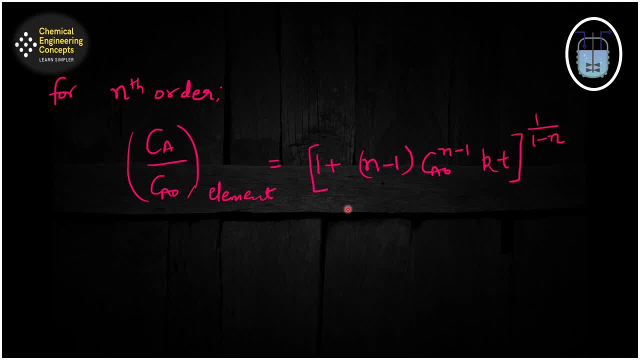 and you will have, uh, you will, you can tackle all the reaction orders for finding out the value of this element. okay, so, because we have, if we have to find out, if we have to find out the average value, we, you know, uh, this value, this value of the each element. 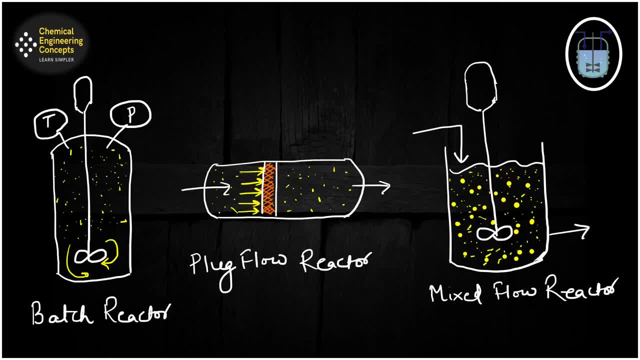 right, and the rtd okay. so both these informations are really very important. so, guys, now let's consider the macro mixing and micro mixing in different ideal reactors. so i have here written the three reactors, three famous reactor, as all you should know. okay, the batch reactor. the plug flow. 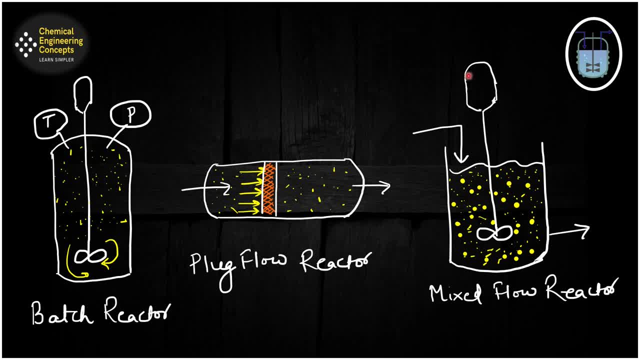 reactor and the mixed flow reactor. so, guys, uh, when it comes to batch reactor, okay, you have, we have taken a simple batch reactor. it is filled with a macro fluid. okay, suppose it is filled with a macro fluid containing the reactant a, any reactant a, since, uh, each aggregate or packet of macro fluid act as its own little batch reactor. okay, 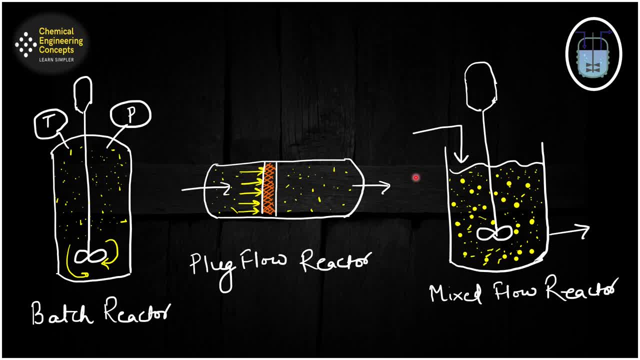 that we already have discussed. the conversion is, in this case, will be same for all the aggregates, because they are spending the same amount of time inside the reactor, and, in fact, we should say that it will be identical with what would you obtain from the micro fluids. okay, so i think. 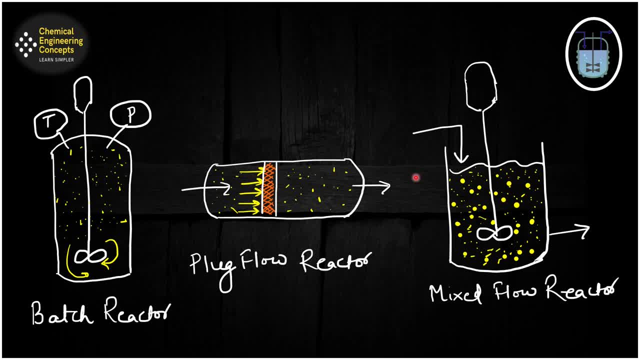 uh, you have got my point here. so the degree of segregation here does not have any effect. okay, so degree of segregation will not affect the conversion, not even the conversion or the product distribution. now let's come to the second type of reactor, that is, the plug flow reactor. 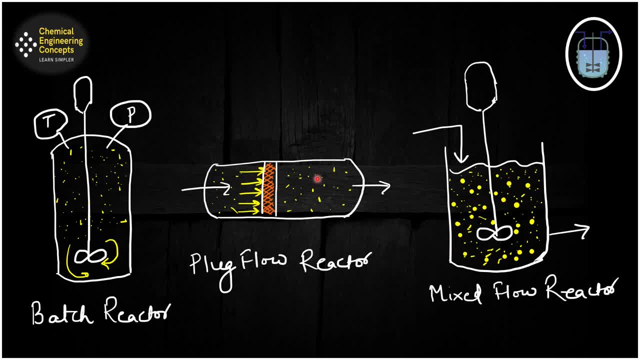 so, since the plug flow can be visualized as a flow of small batch reactors, as i have told you in the beginning of this video, right, that's because we have, like small plugs, okay, plug in the radial direction, so there will be the uh mixing, okay, and they all will act as small batch. 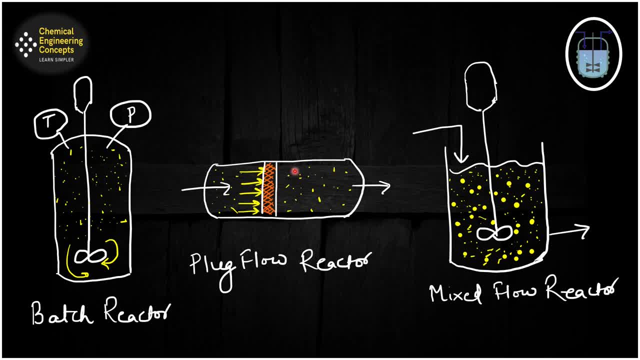 reactors passing in succession through the vessel. so here also the. if the fluid is a macro or micro, that will be. the effect will be alike. okay, there will be no distinct. uh, there will be no difference actually. okay, so the con, the degree of segregation also does not influence in the case of the plug. 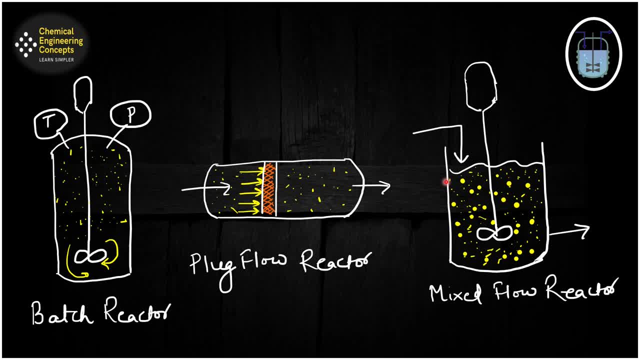 flow reactor. but, guys, when it comes to the mixed flow reactors, you can see, here i have taken both the cases. we have taken the macro fluids, uh, denoted by the large balls, and the micro fluids, denoted by the small balls. so here we shall see both the cases right, the mixed flow reactor with 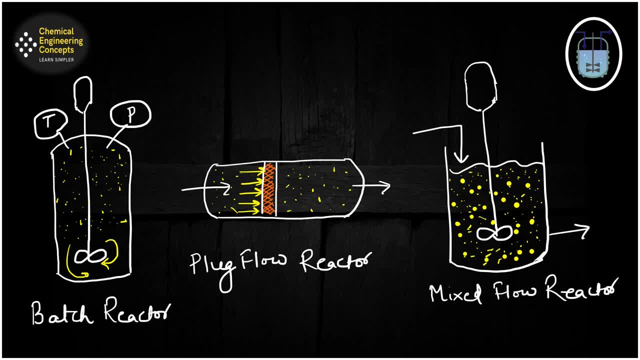 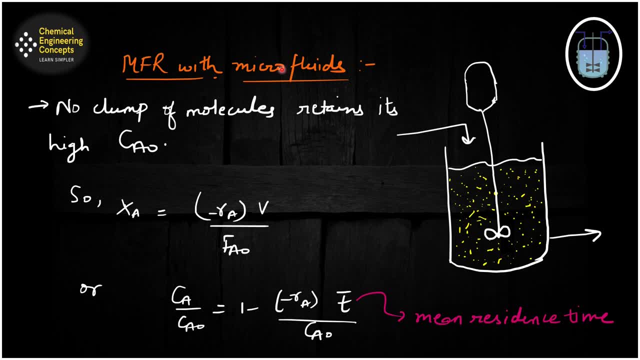 the micro fluids and mixed flow reactor with the macro fluids. so let's jump on to the mixed flow reactor for the micro fluids guys. so here what is happening: when the micro fluids enter the mixed flow reactor, the reactant concentration everywhere will drop to a low value that already 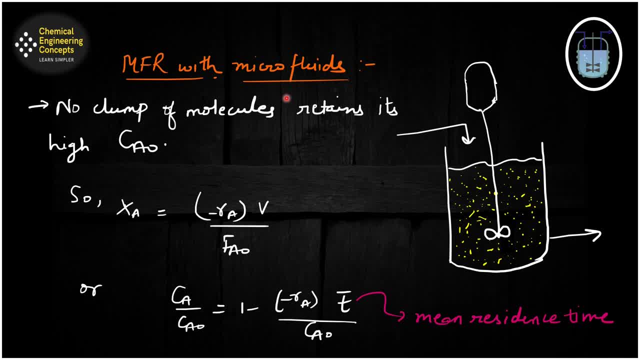 was prevailing inside the reactor and no clump of molecule retains in, retains its- uh, it's a initial concentration, right, and here we may characterize this by saying that each molecule loses its identity, guys. so you should remember this: each molecule is losing its identity and has no. 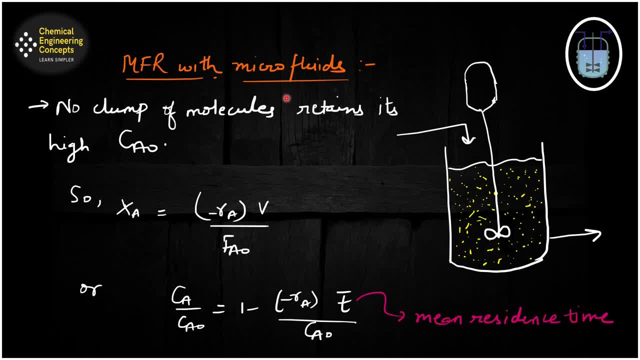 determinable passes right for the case of micro fluids in mfr guys. in other words, we can also say that by examining the different neighbors of each of the molecule we cannot tell whether a molecule is a newcomer or it is. it is an older one, right uh, which is there inside the reactor. so i think 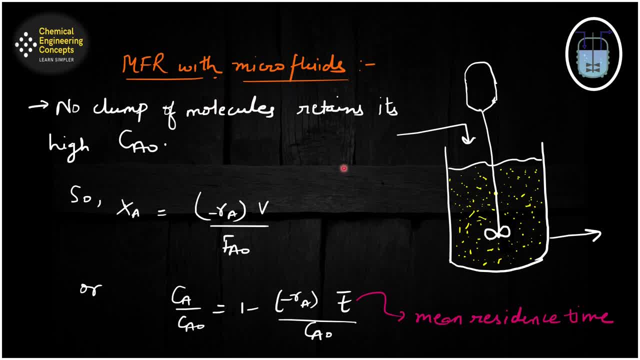 i think here, in this case, uh, since we are not able to, uh, uh, we cannot like distinguish. okay, because since their Highness and all their neighbors are exactly same, so here the conversion will be the same, as we uh determine for the ideal mixed flow reactor right and the concentration. 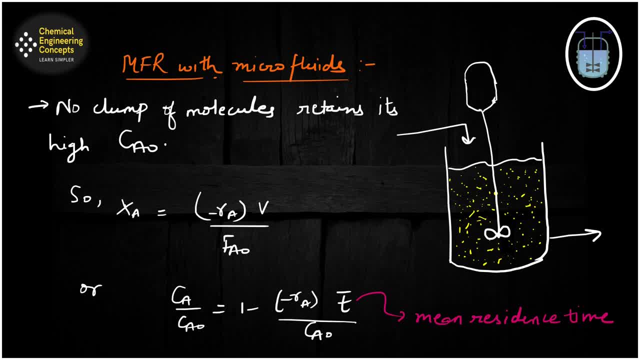 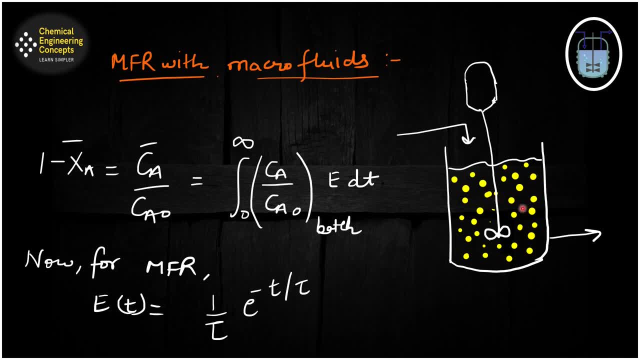 ratio will be the same also, right? so this was the mixed flow reactor with micro fluid. now let's jump on to mixed flow reactor with the macro fluids, guys. so here you can see the macro fluids, the large clump of molecules, right so, flow reactor, the reactant concentration in all the aggregate. we have different aggregates that. 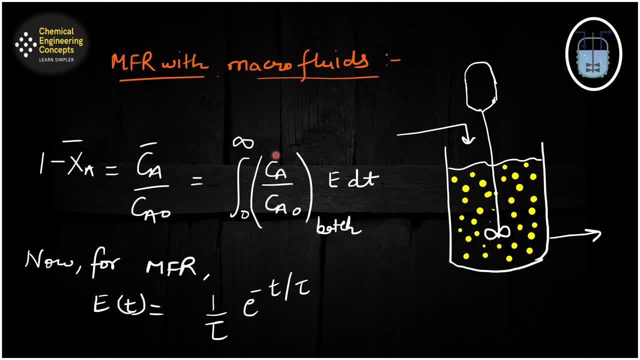 you can see, and the concentration will not be the same, okay, and will. it will drop immediately because it's a mixed flow reactor, but the drops will not be the same. right, this decrease will not be the same because we have different batches. okay, we have different batches and, guys, it's a. 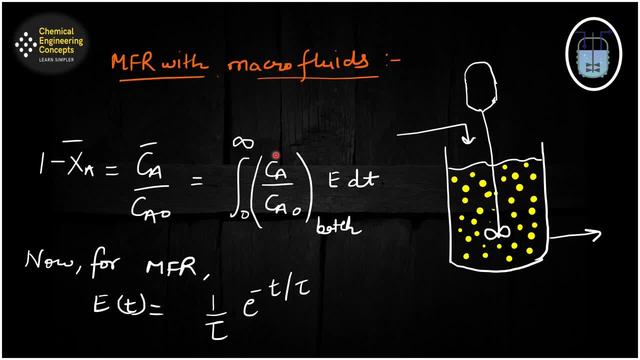 continuous reactor, you should remember this. right? so we have to find out the average. right so we have to take all the batches and we have to integrate from zero to infinite, multiplied by the residence time distribution. right? so we should know these two information. these two information are very important, other than the mixing patterns, right? so first thing is we should. 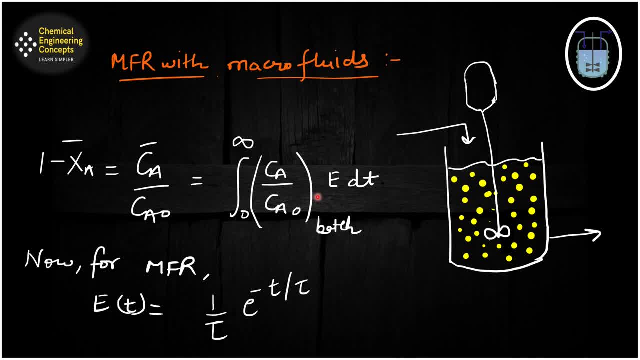 know about the RTD. second thing is about the different batches. okay, we should know the concentration ratio of the batches. and the third important thing is the type of the fluid and the mixing patterns. okay, so both these things are really important. and here this expression: already you know, we have calculated it previously. right now, if I take the RTD function,